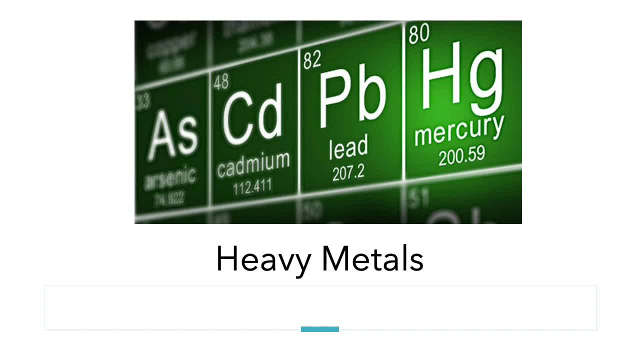 silver and indium, but can be toxic in larger amounts or certain forms. Other heavy metals such as cadmium, mercury and lead are highly poisonous. Potential sources of heavy metal poisoning include the mining, tailings, industrial wastes, agricultural runoff, occupational exposure, paints and treated timber, Chromium, arsenic. 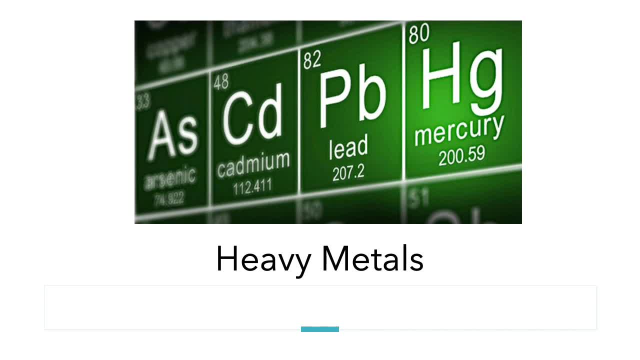 cadmium, mercury and lead have the greatest potential to cause harm on account of their extensive use, the toxicity of their combined form or elemental form and their widespread distribution In the environment. we'll be limiting our discussion to three: the arsenic, lead and mercury. 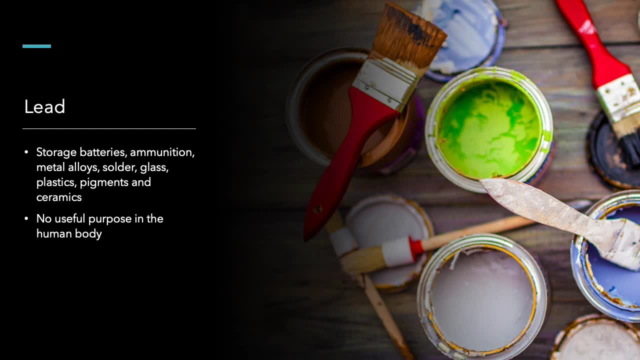 Lead is one of the oldest and most prevalent heavy metal contaminants in the world, Once ubiquitous in nature, but due to many public health measures and policies, the use of this has declined significantly. Lead can be found in storage batteries, ammunition, metal, alloys, solder, glass, plastics, pigments. 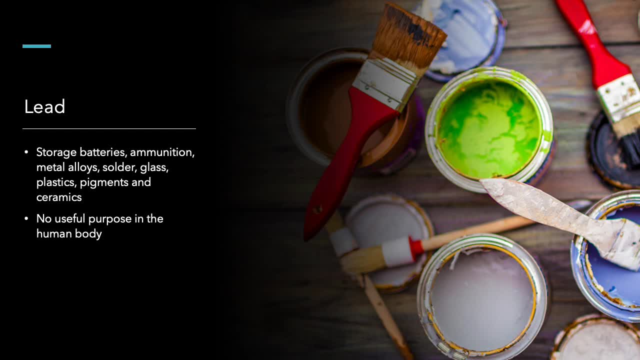 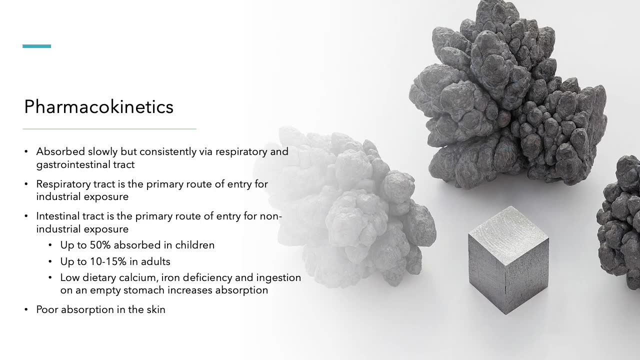 and ceramics. As of today, there are no useful purposes for this in the human body. What are the important pharmacokinetic profiles of lead? Lead is absorbed slowly but consistently via respiratory tract and GI tract. Respiratory tract is the primary route of entry for industrial exposure Intestinal. 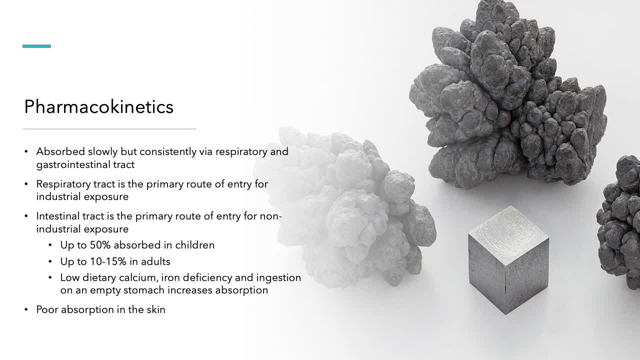 tract, on the other hand, is the primary route of entry for non-industrial exposure or at homes. Up to 50% can be absorbed in children. However, only up to 10 to 15% is absorbed by adults. The low dietary calcium and iron deficiency and ingestion on an empty stomach increases absorption. 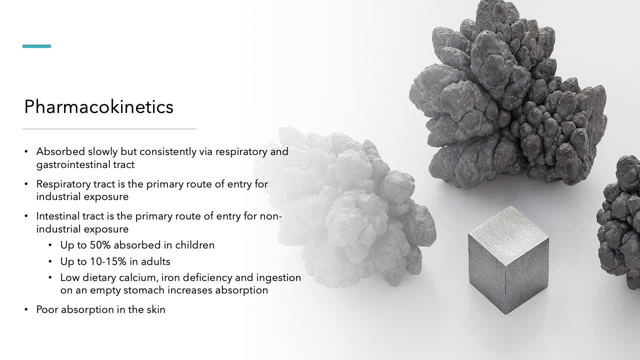 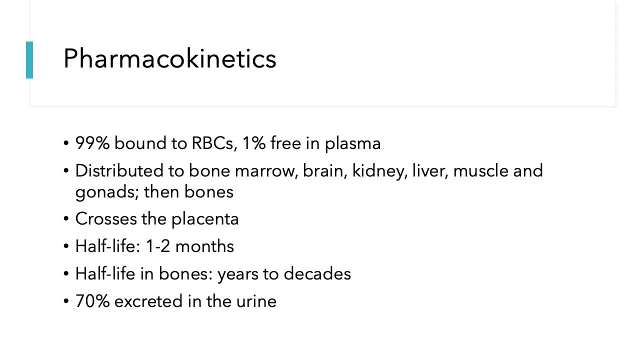 of lead. Fortunately, lead has poor absorption in the skin. Once it enters the bloodstream: 99% is bound to RBC or erythrocytes, 1% free in plasma. The distribution starts from soft tissues to hard tissues like bone, as follows: from bone marrow: 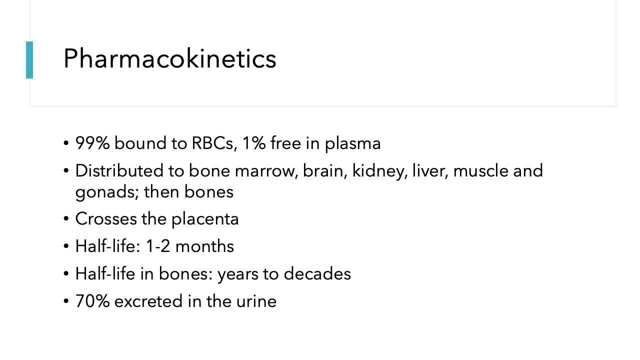 to the brain, to the kidney, liver, muscle and gonads and then to the hard bones. It has the ability to cross the placenta. The half-life is 1 to 2 months. However, when it is inside the bones, it may take years to decades before it gets cleared from the bones. 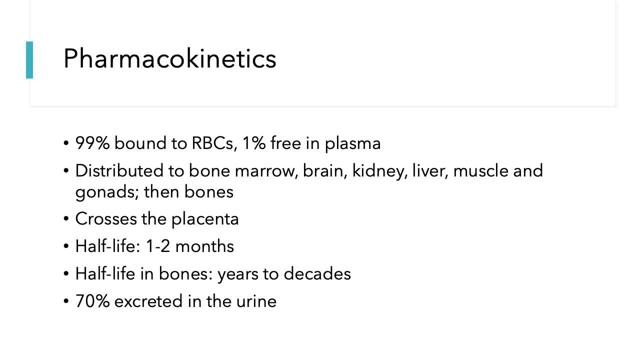 This slow-release response by the lead in the bone may produce symptoms for years on. some patients who've been exposed to lead, Like, for example, patients who had gunshot wound where the bullet was not or never removed from the body, There were reports. 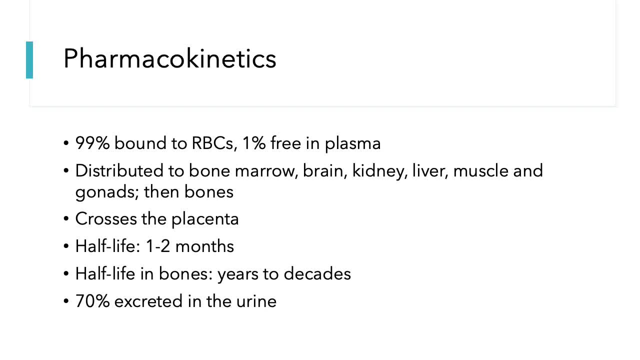 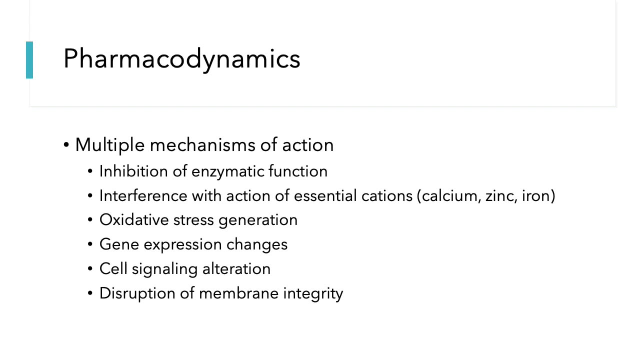 that they developed lead intoxication over a few years. 30% of lead is excreted in bile, skin, hair and nail, while 70% is excreted in the urine. Like some of the heavy metals, they have multiple mechanism of actions. 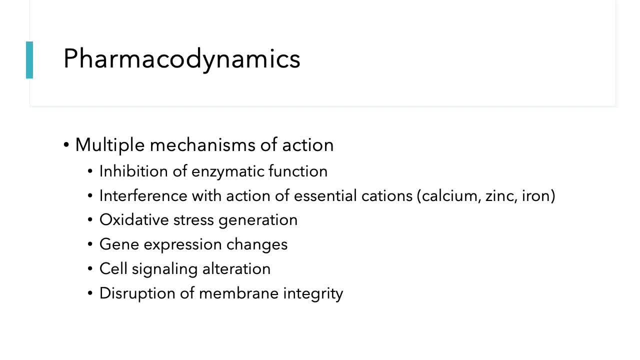 First, they inhibit enzymatic function. They interfere with essential cations like calcium, zinc and iron. They produce free radicals- radicals or oxidative stress. They have ability to change gene expression, They alter cell signaling mechanisms and they disrupt membrane integrity. 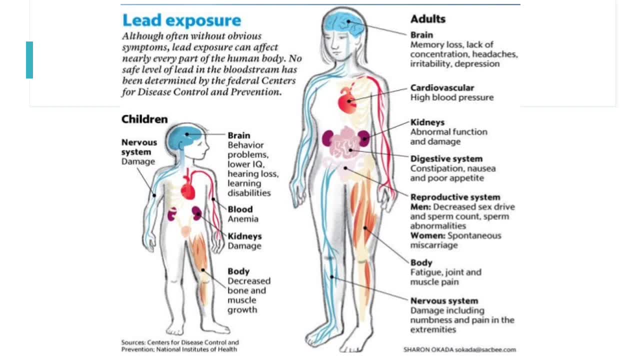 Although often without obvious symptoms, lead exposure can affect nearly every part of the human body And, as of today, there is no established safe level in the human blood for this heavy metal. What are the different effects to the different organs of lead In the CNS or central nervous system? the developing brain of a child and fetus is the most. 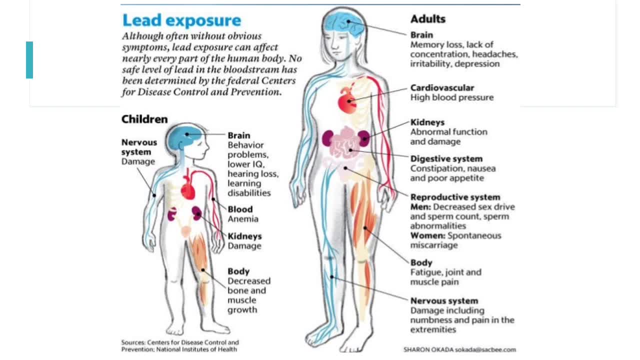 sensitive target organ for lead Effect may include behavioral problems, lower IQ, hearing loss and learning disabilities. In adults the CNS is less sensitive, but prolonged exposure may have behavioral and neurocognitive effects. In the blood it may produce normocytic, microcytic or hypochromic anemia. Lead interferes with the 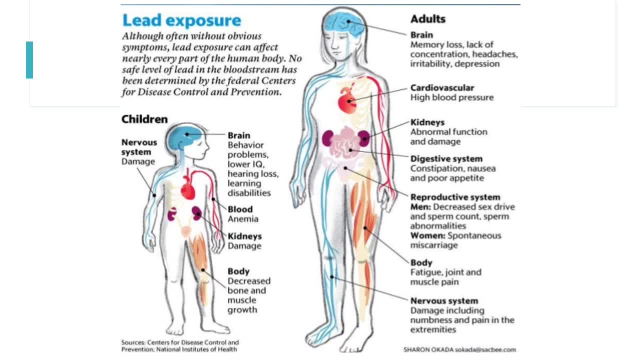 heme synthesis by blocking the incorporation of iron in protopyrine 9 and by inhibiting enzymes in heme synthesis. The renal, the chronic high-dose exposure may lead to renal interstitial fibrosis and nephrosclerosis In the reproduction or reproductive organs. high-dose exposure. 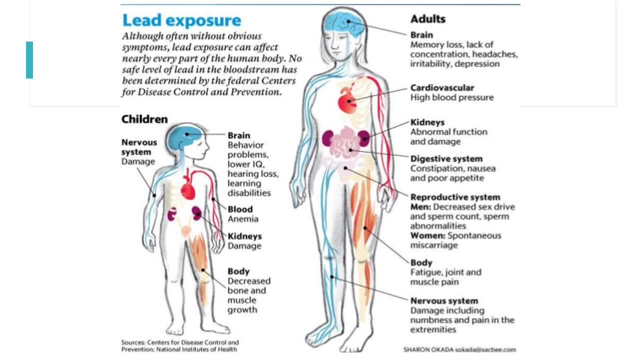 may lead to stillbirths or spontaneous abortion. GI tract Patients may develop intermittent or severe colicky abdominal pain, also called lead colic. Other symptoms may include loss of appetite, constipation or diarrhea. In the cardiovascular, it has been linked with increase in both systolic 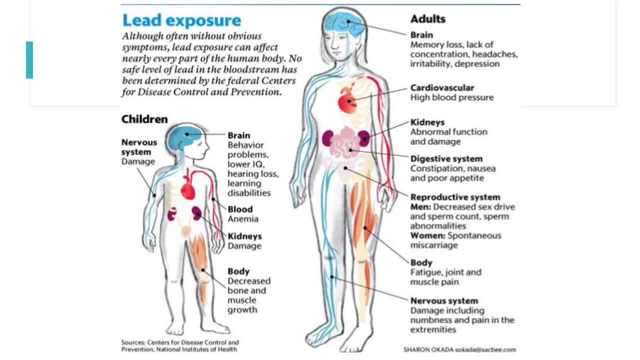 and diastolic blood pressures in multiple studies, Also with QT interval prolongation. the Mysteriosver, reporting an increase in lead production despite it, was rated as a minor tranfer. 1. Blood levels at about 10-25 yerde per deciliter, arguably understandably lower than any other. 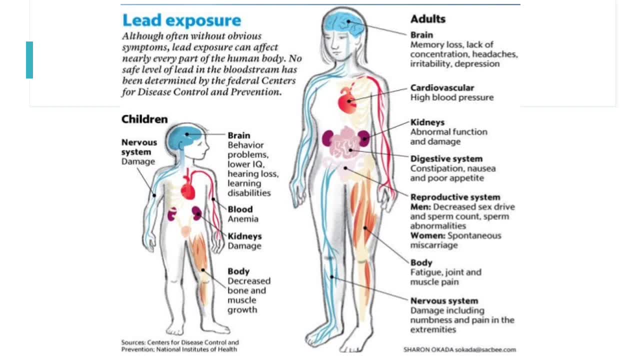 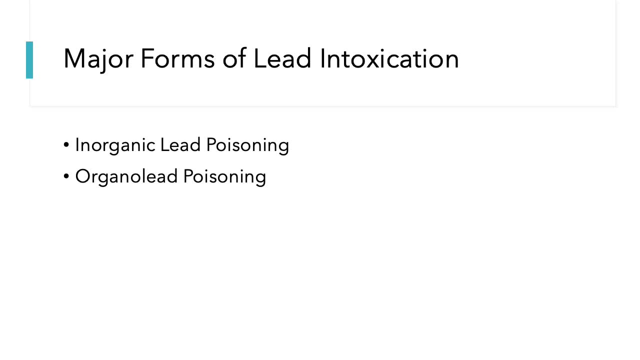 drug in America showed at blood blood level of 10-25 Fold 8. 1.. at blood levels at about 10-25 micron per deciliter, significant cardiovascular mortality has been linked. Although prevalence in the US has since decreased, still a major problem in other parts of the globe. There are two major forms of lead intoxication: those that are caused by inorganic lead and those that are caused by organic lead. 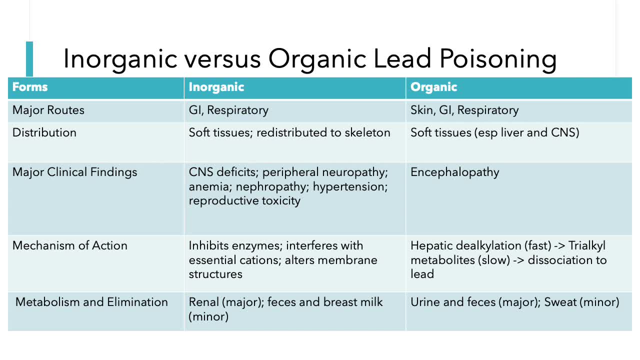 are the difference between inorganic lead poisoning and organic lead poisoning. In organic lead poisoning, the major routes are GI and respiratory tract. The distribution starts from soft tissues, as I've mentioned in the previous slides, and then it gets redistributed to the skeleton. Because of its wide distribution and multiple mechanism of actions, there's a lot of 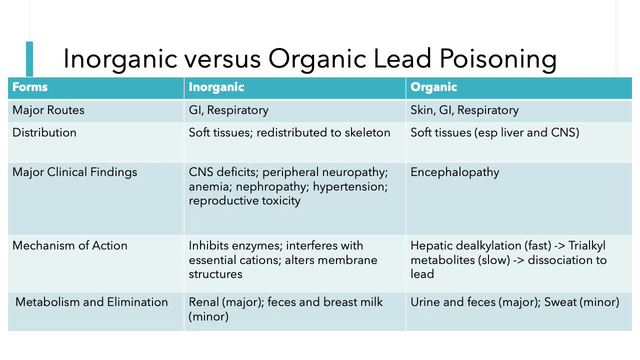 clinical findings that you can see in inorganic lead poisoning, like CNS deficits, peripheral neuropathy, anemia, nephropathy, hypertension, reproductive toxicity. The metabolism and elimination route of this is in the renal or in the kidney, and some can be eliminated by 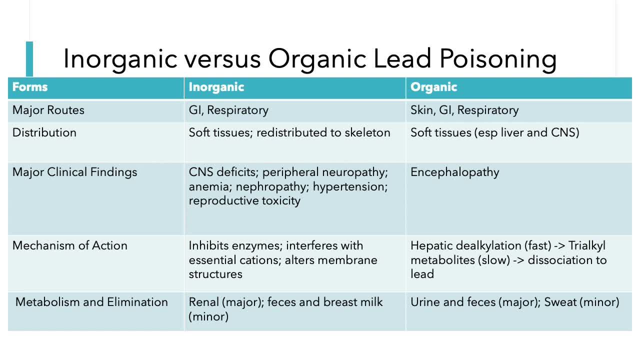 feces and breast milk as well. So organic lead poisoning is very rare now because of the public health measures we've undertaken to prevent its use in the environment and in the incubation Before it is found in gas as tetraethyl and tetramethyl lead. In some areas, though, 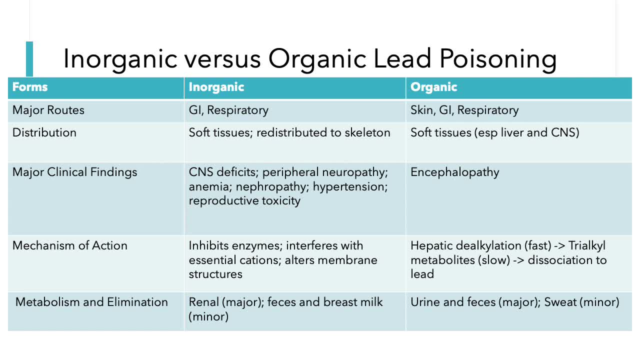 it's still used as lead stearate and lead naphthenate. The major routes for this are skin, GI, respiratory, and the distribution is limited to soft tissues, with preference for liver and CNS. The major clinical finding is encephalopathy and sometimes hepatotoxicity. The mechanism of 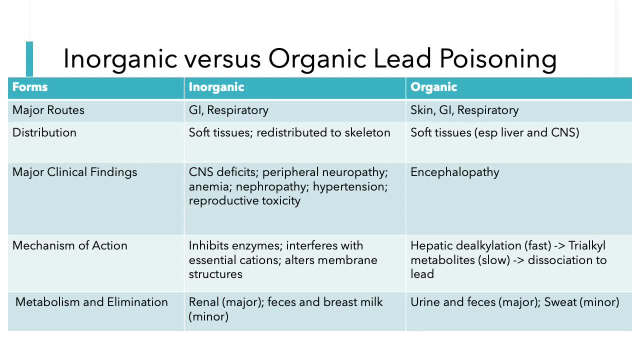 action is: first it undergoes the alkylation in the liver to become triacheal metabolites and then they're dissociates into lead. The metabolism and elimination pathway is primarily from the urine and the feces, and sweat is a minor route. 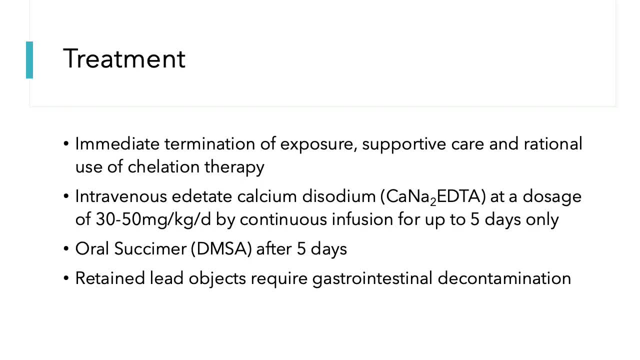 of excretion. Before we go to treatment we have to emphasize that for these heavy metals we need to reduce or prevent excessive exposure, especially in homes, in the environment and in the workplace. So the cornerstone of treatment are three: immediate termination of 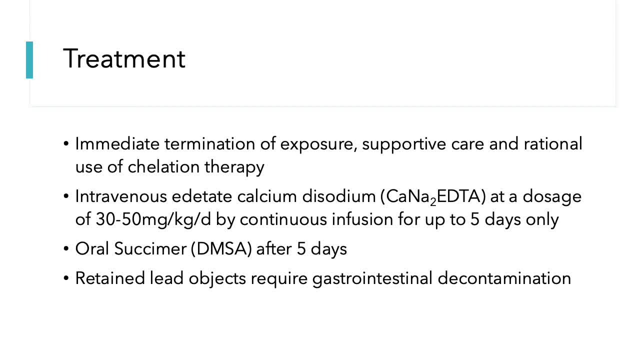 exposure. that's very important. supportive care, whether they're intensive or regular supportive care, and the rational use of chelation therapy, which we will discuss later as well. The intravenous EDTA, or EDETATE calcium disodium, at dose of 30 to 50 milligram per kilogram per day. 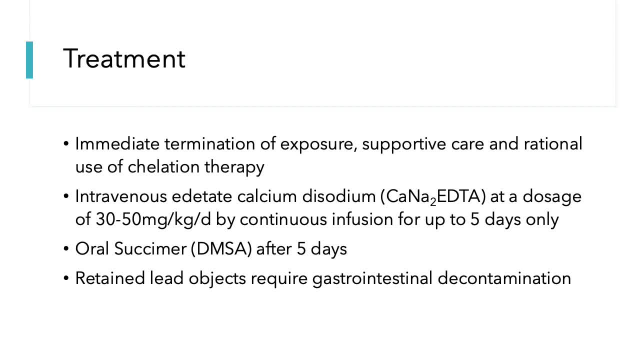 by continuous infusion for up to five days only, And then it will be followed by oral succimer or DMSA after five days if the treatment remains to be incomplete. Some patients, like patients presenting with lead encephalopathy, may require: 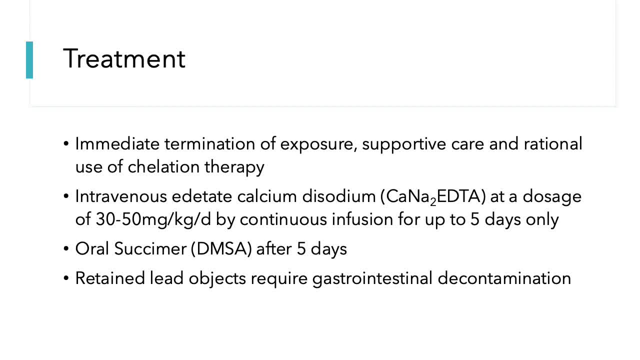 intensive care as well. Cerebral edema may be given with steroids, mannitol or hypertonic saline Anticonvulsants. if patients start developing seizures as well, Retained lead objects like in the GI tract or some gunshot wound require decontamination. 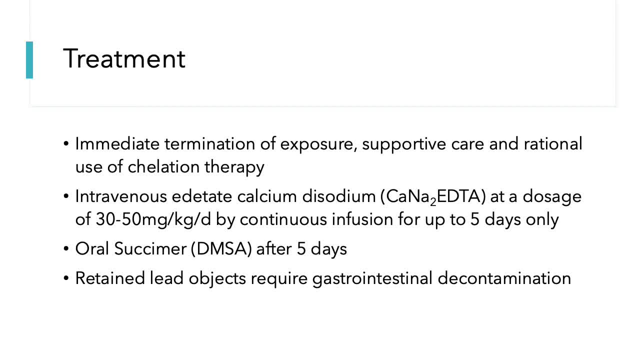 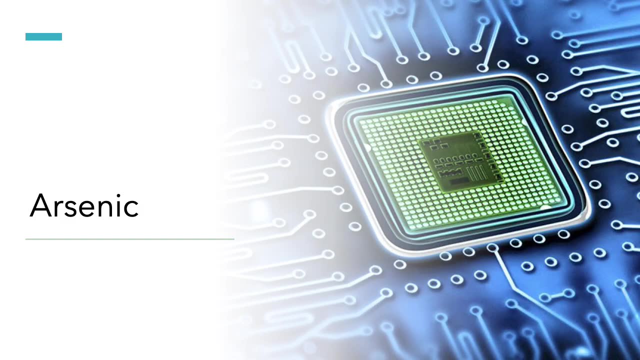 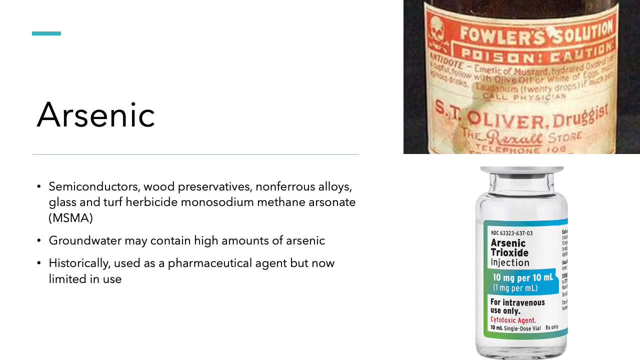 So the end point or objective of therapy is the resolution of symptoms or return of blood lead concentration to pre-morbid range. Let's now go to arsenic, found mainly in semiconductors and many other products in the manufacturing industry. So arsenic is a naturally occurring element in the nurse's crop. 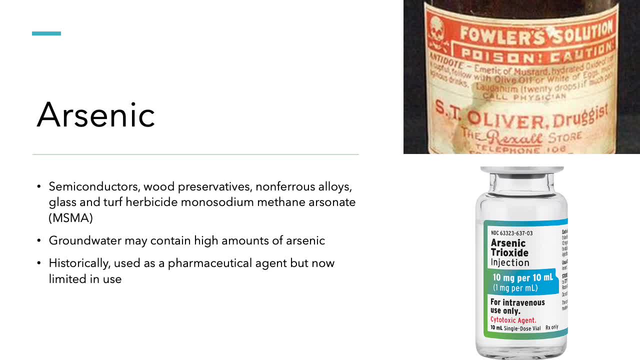 So arsenic is a naturally occurring element in the nurse's crop. So arsenic is a naturally occurring element in the nurse's crop. It provides a bomscnya condensate to some souls, coraz, with a long history of use as a constituent of commercial and industrial products. 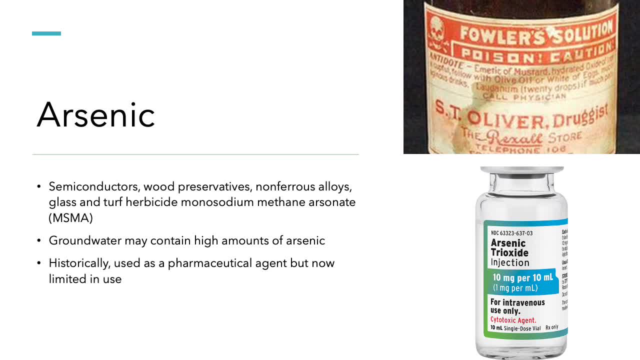 and as a component on some pharmaceuticals, like our Fowler's solution before, And as an agent of deliberate poisoning, and in recent commercial applications such as the muito. No insights out of the product. il contenit ur 현재, perfectly oiled, and the miniaturin that it is used for. 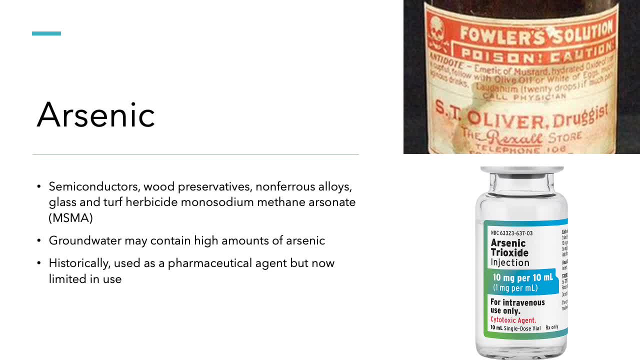 abide by standard상 ما ellos carry a percentile slowing move's rate if a particular site has been inexpensively 僵. Medicines aretype of industrial applications like laid-up stem or silica, non-ferrous alloys or seed oil. It has anti-那个 짜 участок. nasal kiplait sama張hia di agung. Sorry for the biết. ngayor tetanus and 125 dirhams digested yureng- tengahqi prodkars. 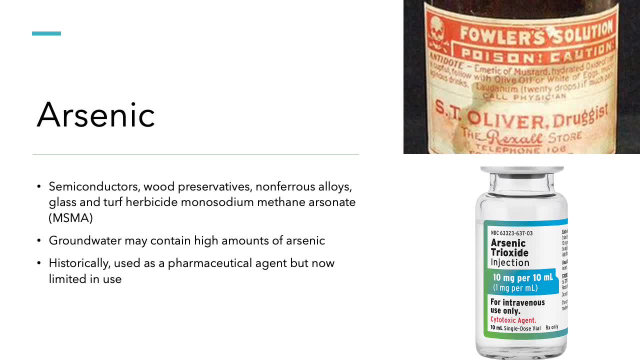 monosodium, methane, arsenate or MSMA. In some regions of the world, groundwater may contain high levels of arsenic that has leached from the natural mineral deposits. Arsenic in drinking water in the Ganges Delta of India and Bangladesh is now recognized. 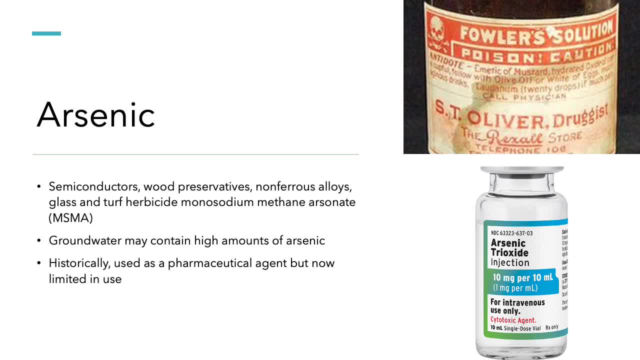 as one of the world's pressing environmental and public health problem to date. It is of historical interest that before there's such a thing, what they call Fowler's Solution, Which contains one potassium arsenite, It was widely used as a medicine for many conditions. 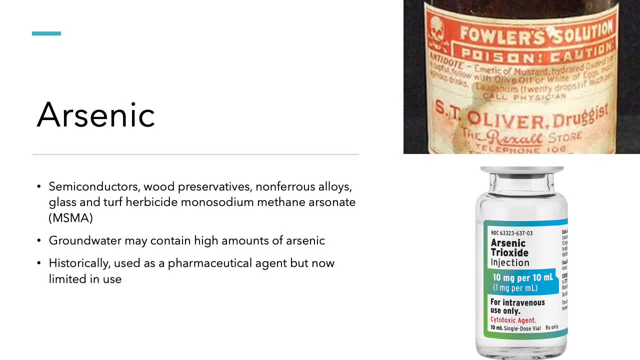 in the 18th century through the mid-20th century. Organic arsenics were the first pharmaceutical antibiotics or antimicrobials and were widely used for the first half of the 20th century until it was supplanted by sulfonamides. 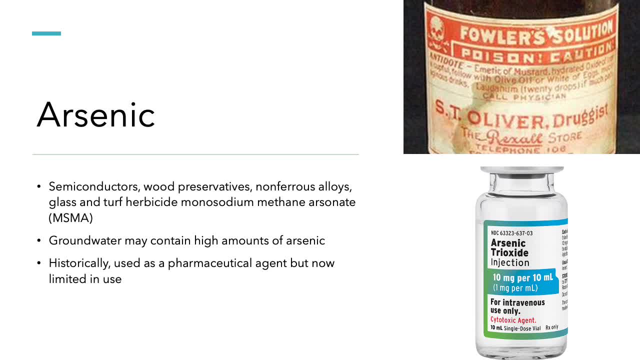 and other more effective and less toxic agents. So Fowler's agent was invented by Thomas Fowler. He used it to make and use this to treat a variety of ailments, including asthma, chorea or eczema, pempigus, psoriasis, Hodgkin's lymphoma and leukemia. 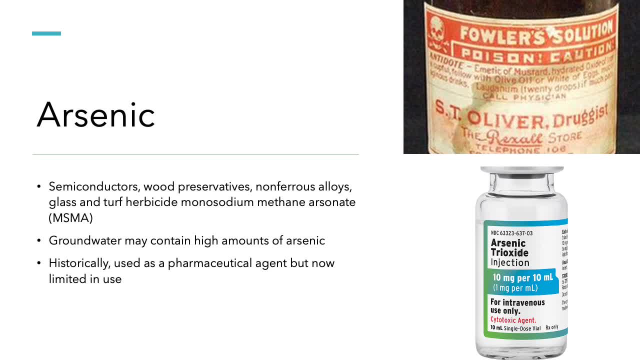 Because of its multiple side effects by the 20th century, including cirrhosis of the liver, idiopathic portal hypertension, urinary bladder cancer and skin cancers, the solution's popularity diminished And now it's banned for use. However, in 2000, it was introduced as an orphan drug. 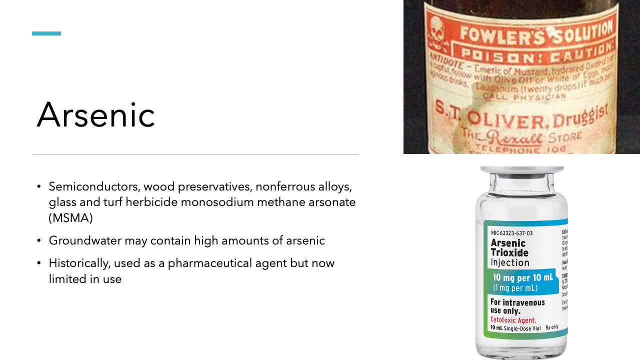 for treatment of relapsed acute promyelocytic anemia in the form of arsenic trioxide injection. So that's the only accepted use. FDA approved for relapsed acute promyelocytic anemia And metamilarsoprol, another drug that has arsenic. 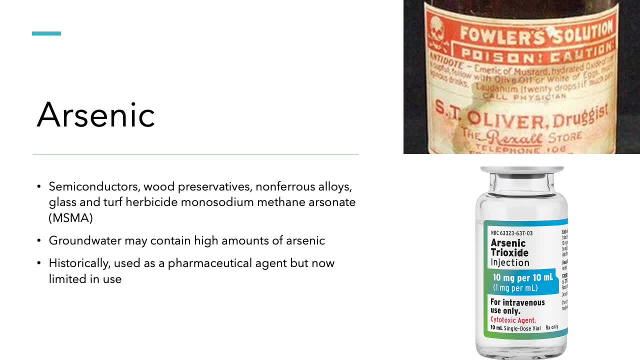 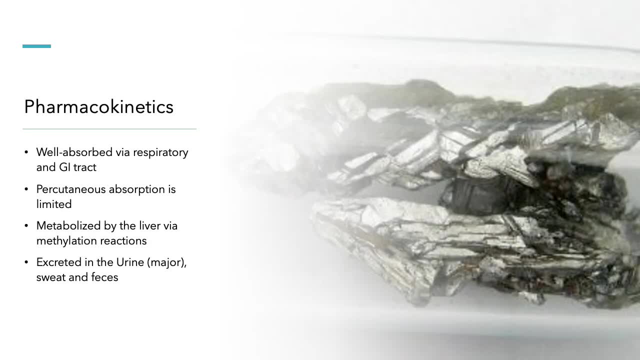 is used for treatment of African type anemia, Like cel, journeyategory 10, and epinephrine. the only one that worked in the public eye File of arsenic is that it's well absorbed by the respiratory and GI tract. 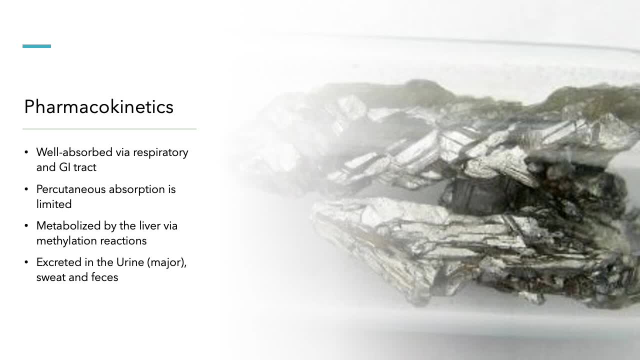 It has limited percutaneous or skin absorption. It is metabolized by the liver via methylation reaction. It is also excreted in the urine. Please take note that although the absorption in the skin is limited but clinical significant, the absorption is very limited. 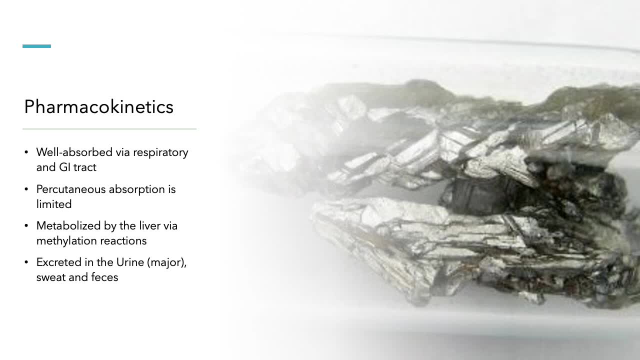 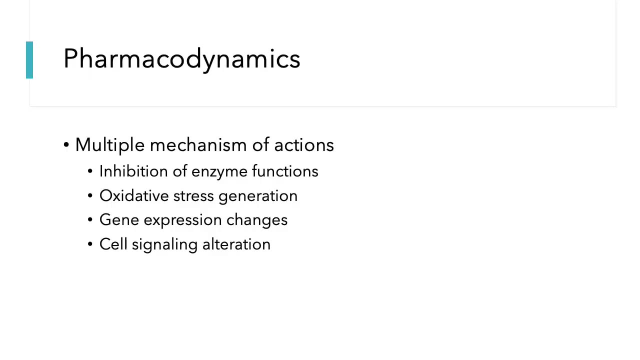 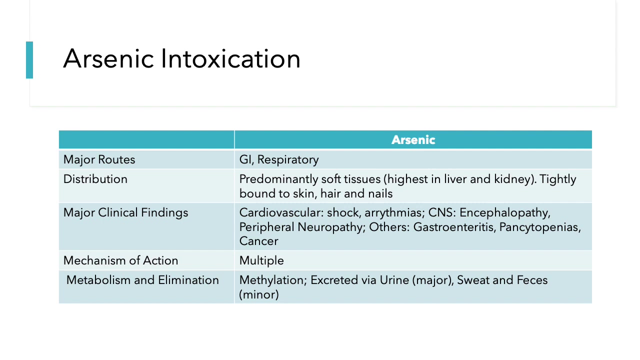 These effects are also observed during heavy exposures. Again, it shares multiple mechanism of action, like inhibition of enzyme function, oxidative stress or free radical generation, gene expression alteration, cell signaling changes. This is just a summary of arsenic intoxication that we've discussed in the previous slides. 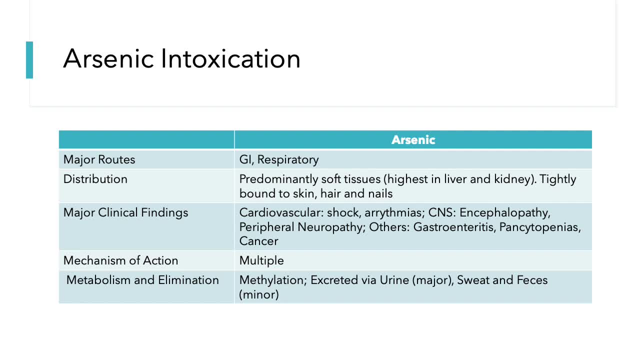 The major clinical findings that you can see in arsenic intoxication are cardiovascular shock arrhythmias, CNS. we have encephalopathy, peripheral neuropathy as well. Others have gastroenteritis, pancytopenia And multiple forms of cancer. 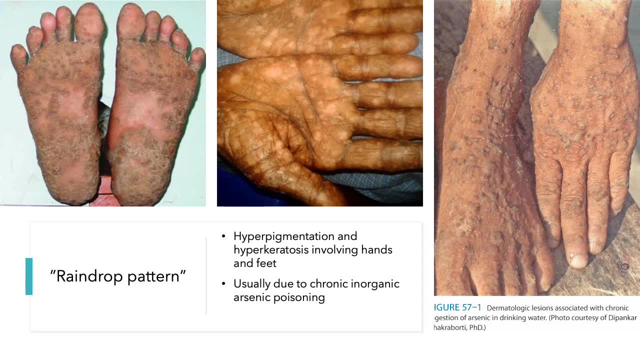 One characteristic finding in chronic inorganic arsenic poisoning is what we call a raindrop pattern in the skin. Skin changes is among the most characteristic effect. typically develops after years of exposure. Raindrop pattern, as you can see in the pictures, are patterns of hyperpigmentation. 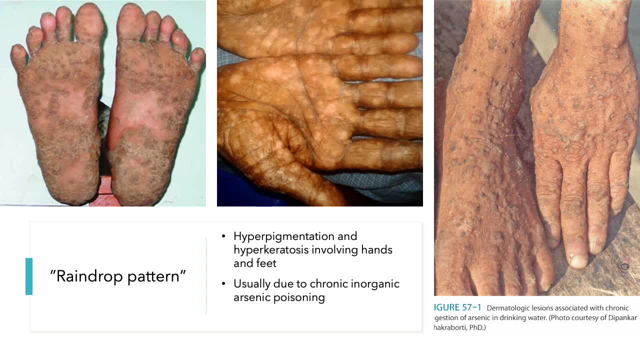 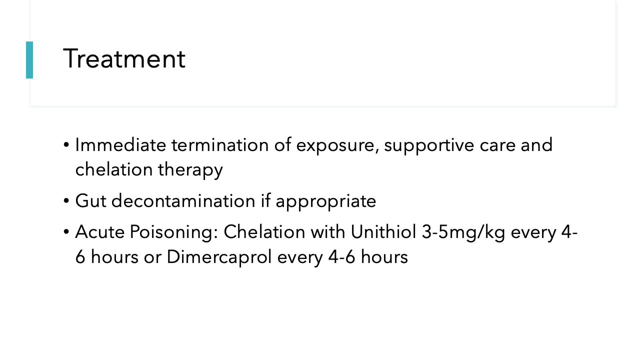 And in keratosis involving the hands and the feet. The cornerstone of treatment in immediate termination of exposure. supportive care, whether they're intensive or regular supportive care, and chelation therapy: Gut decontamination. if needed And for acute poisoning, the choice is chelation with unitile 3-5 mg per kg every 4-6 hours. And for acute poisoning, the choice is chelation with unitile 3-5 mg per kg every 4-6 hours. And for acute poisoning, the choice is chelation with unitile 3-5 mg per kg every 4-6 hours. 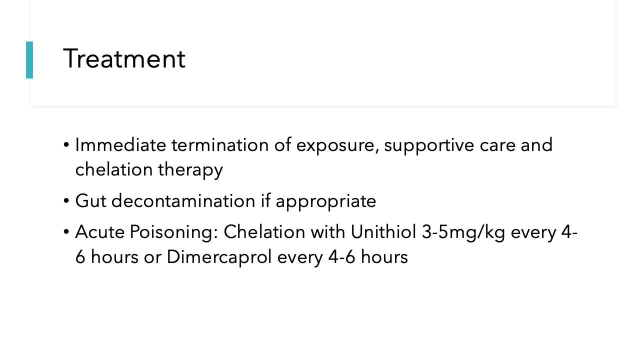 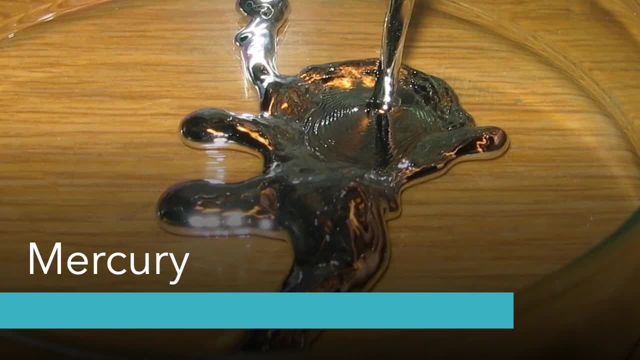 Or dimer caprol every 4-6 hours. Now, the last is the most famous of them all. probably you know: mercury, The liquid metal or also known as quicksilver- We've probably heard of this in the news- when DOH closes down schools or facilities when there's mercury spill. 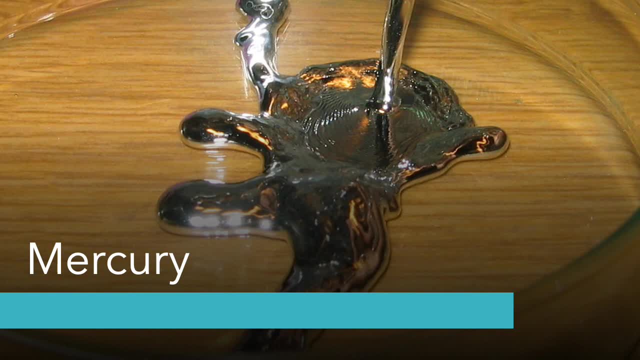 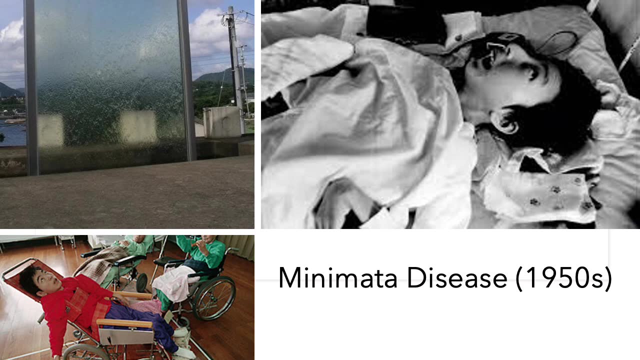 Why is this done and why is it important? in 1950s there was this incident called minimata's disease, secondary to mercury poisoning. so what happened in minimata's disease? in the early 1950s, resident of minimata, small coastal city in southern japan, began observing some startling animal behavior. first, now, cats would suddenly. 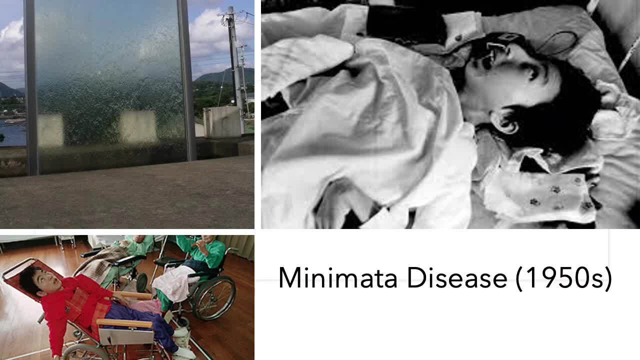 foam in the mouth, and then dogs as well. birds would crash land, fish would inexplicably go belly up. before long, humans too were suffering from what became known as minimata disease. patients developed slurring of speech, stumbling about and having trouble with simple tasks such as buttoning buttons. the culprit finally emerged in 1959, when it was determined: 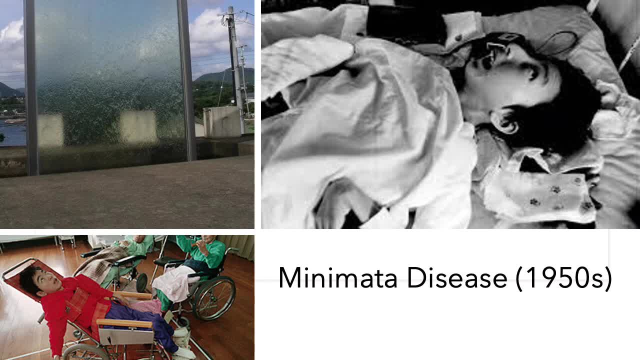 that the chemical company chiso corporation, one of minimata's biggest employers, was dumping mercury in the sea as part of its manufacturing process and that this toxin was poisoning people and animals as well were local who ate local seafood. chiso continued releasing mercury tainted water until 1968, reportedly causing at least 2 000 more deaths, as well as 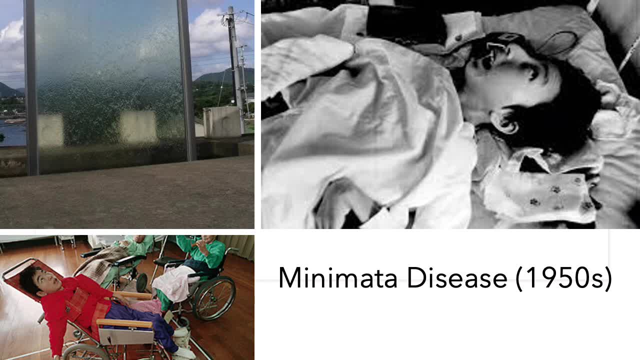 birth defects, paralysis and other maladies. in commemoration of the minimata disease, in 2013, the, under the international minimata convention, 128 countries committed to the worldwide phase out of, by 2020, of mercury. philippines is one country who signed this into law as well. 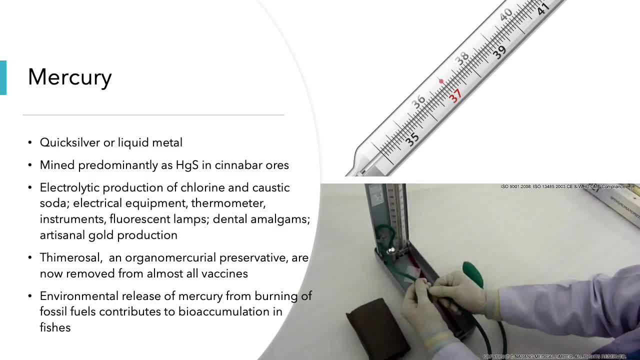 mercury is also known as your quicksilver, or liquid metal, because it is the only metal that is liquid in ordinary conditions or temperature. today it has been largely removed in the instruments like bp apparatuses and thermometers, but we still encounter them in sub folk medicine, antiseptics and cosmetic. 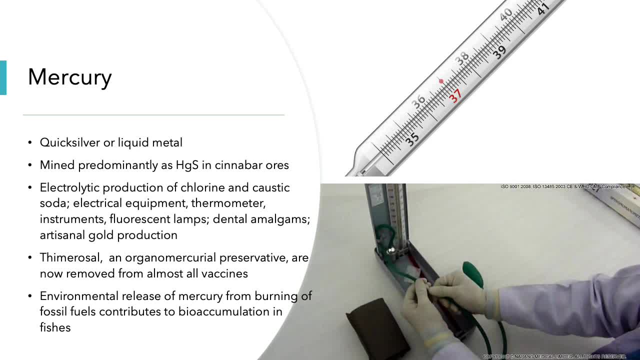 skin lightening products, the unregulated ones. it is mined predominantly in cinnabar ores. it was also found in electrolytic production of fluorine and caustic soda, electrical equipment in thermometer instruments, fluorescent lamp, dental amylose料. Islam also found in electrolytic production of chlorine and caustic soda, electrical equipment and thermometer instruments, fluorescent lamp, dental amylose, levafe, et cetera. 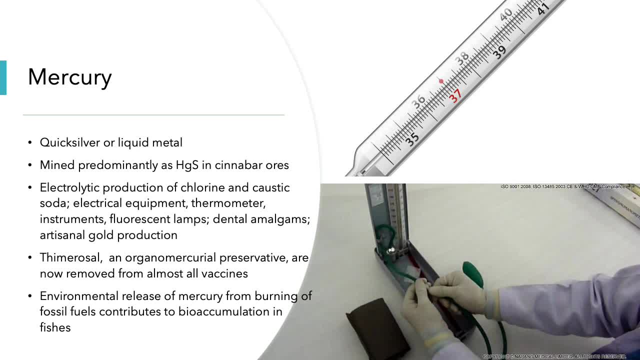 GAMs are traditional gold production. Timerosal, once found in vaccines, an organomercurial preservative, are now removed from almost all of the vaccines. because of this, Environmental release of mercury from burning fossil fuel contributes to the bioaccumulation in fishes. 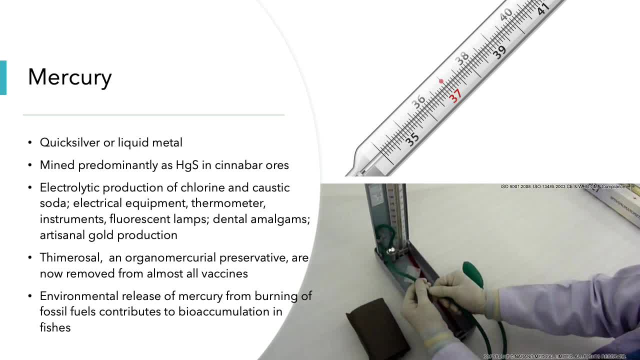 Again in 2013,, under the Minamata Convention, 128 countries committed to the worldwide phase out by 2020 in numerous products like thermometers, pesticides and batteries, And by 2025, it is banning this as well in manufacturing process, like your chloral alkali. 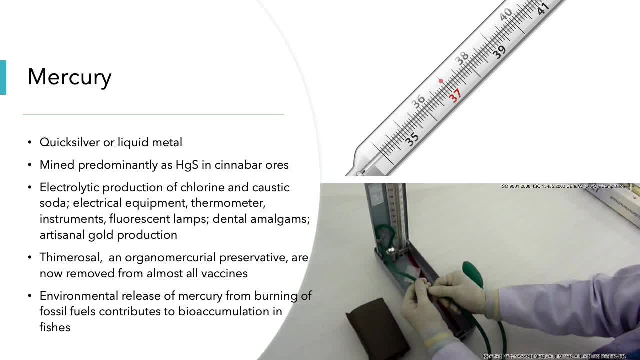 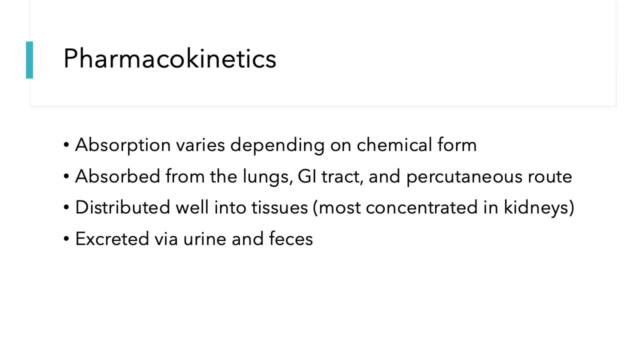 production. Philippines is one of the countries who signed this Minamata Convention. Inhalation is one of the major occupational sources of mercury poisoning. Absorption varies depending on the chemical form, and usually it's absorbed from the lungs, GI tract and the skin. 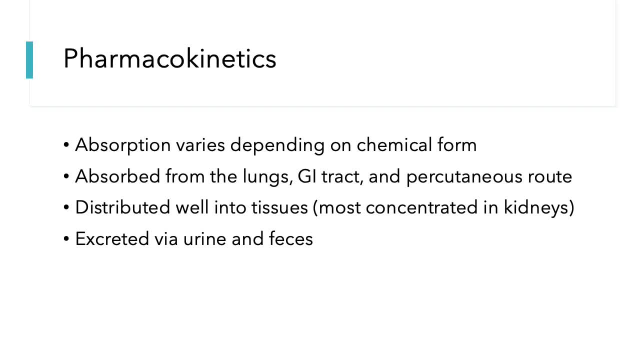 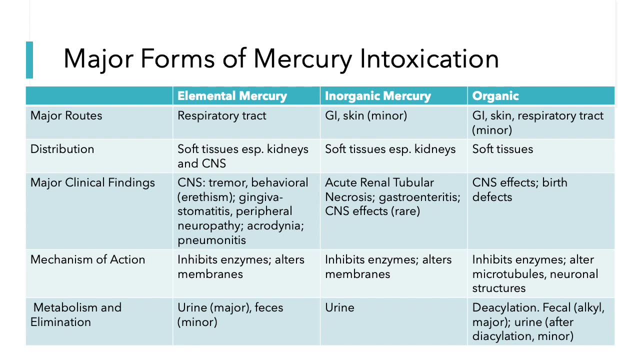 It is distributed well into tissues and mostly concentrated in the kidneys. Therefore, a fraction of this is retained in the kidney- and also in the brain as well, for months to years. It is excreted via urine and feces. There are three major forms of mercury intoxication. 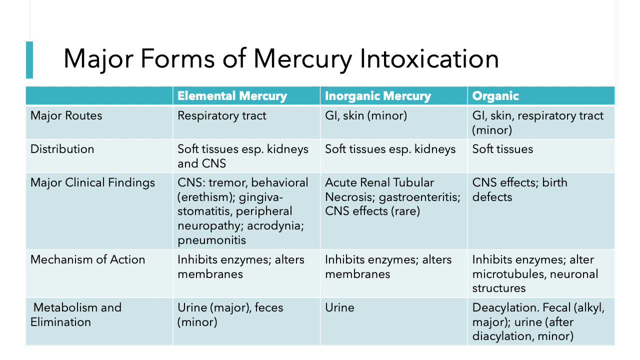 The elemental mercury, inorganic mercury and organic mercury, intoxication or poisoning. So let's first discuss elemental mercury. It's usually taken up by a respiratory tract distributed from soft tissues, especially the kidneys and the CNS. The major clinical findings are tremor, behavioral changes or what you call erythesim. erythesim- 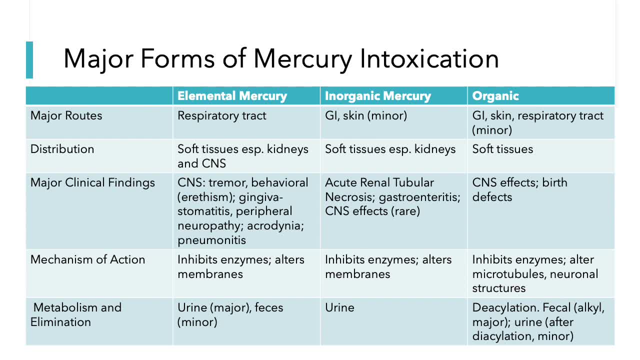 mercuralis Or Mad Hatter's disease. It's a neurological disorder presenting with behavioral changes such as irritability, low self-confidence, depression, apathy, shyness and timidity, And in some extreme cases, with prolonged exposure, it may also cause delirium and personality. 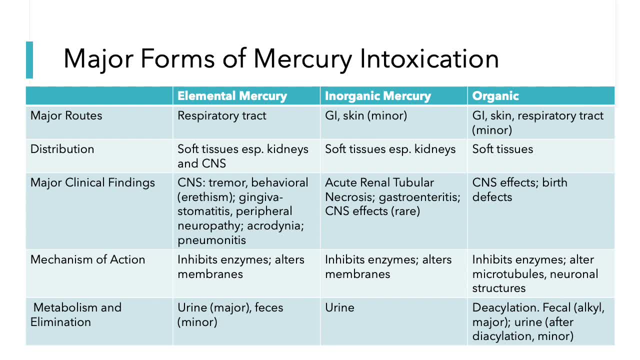 changes and memory loss. So other symptoms are gingival somatitis, peripheral neuropathy, acrodinia and pneumonitis. The mechanism of action is two: inhibits enzymes and alters membranes. The major route of elimination is urine and minor via feces. 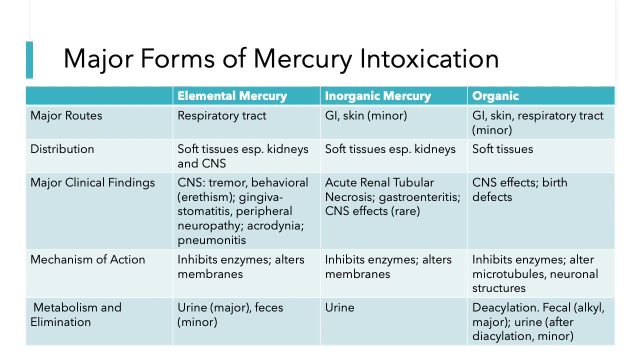 Inorganic mercury, on the other hand, can be absorbed in the GI and in the skin as a minor route. Soft tissues are again affected by this and has preference for kidneys. Therefore, the major clinical findings are acute trigonal tubular necrosis. 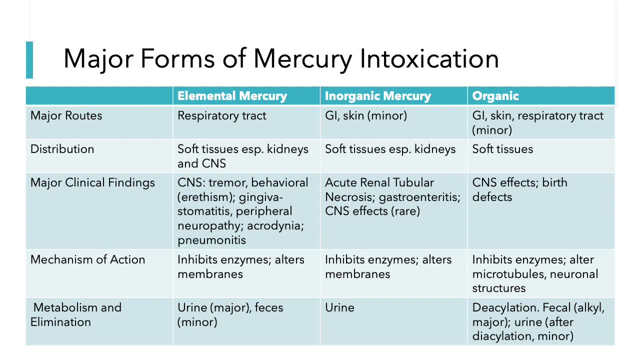 Some patients also develop gastro Enteritis, and CNS effects are very rare, although seen as well. The mechanism of action is: the inhibits enzymes alters membrane and then it is eliminated via urine. Organic, on the other hand, has three routes: GI, skin and respiratory tract. 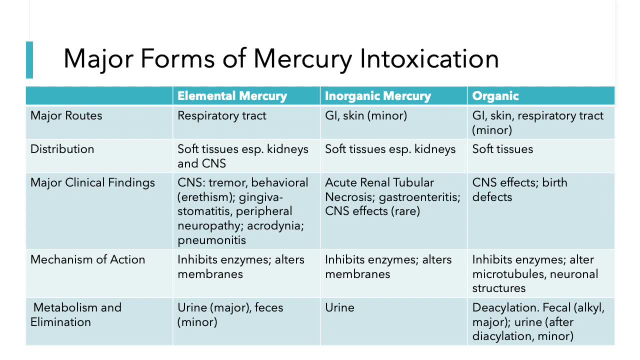 The distribution is limited to soft tissues, with no preference whether to kidneys or CNS, So it's distributed well all throughout. The major clinical findings are CNS and birth defects. The mechanism of action: they inhibit enzymatic action. alteration of microtubules or neuronal structures. 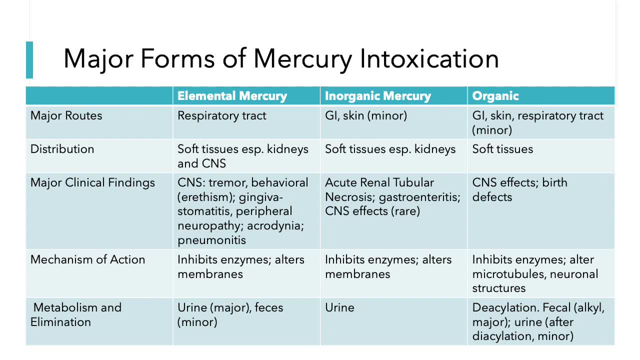 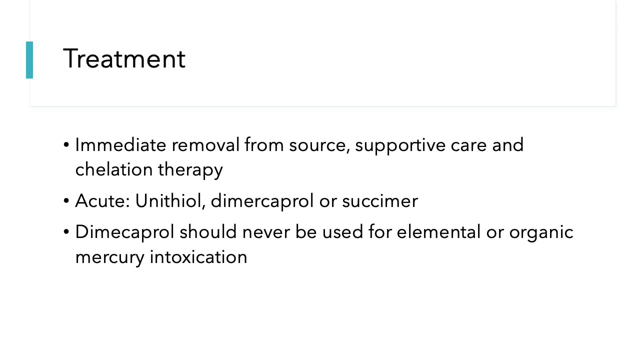 The metabolism and elimination routes are the isolation in the liver and fecal elimination. Some parts go to the urine as well. The cornerstone of treatment is the same as the previous previous two heavy metals. you immediately remove the patient from the source. you provide supportive. 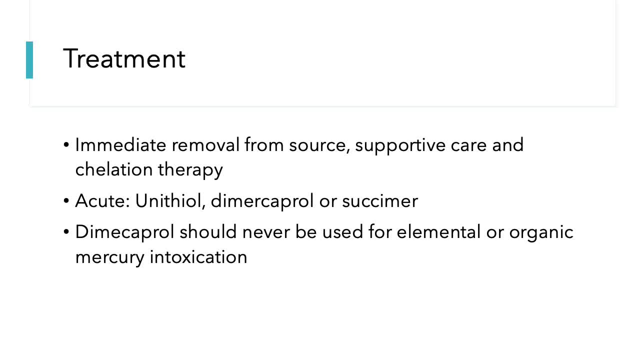 care and then chelation therapy. The acute phase is treated with unitile dimercaprol or succimer. However, dimercaprol should never be used for elemental or organic mercury intoxication because of redistribution. So we will talk about that redistribution later in chelation therapy. 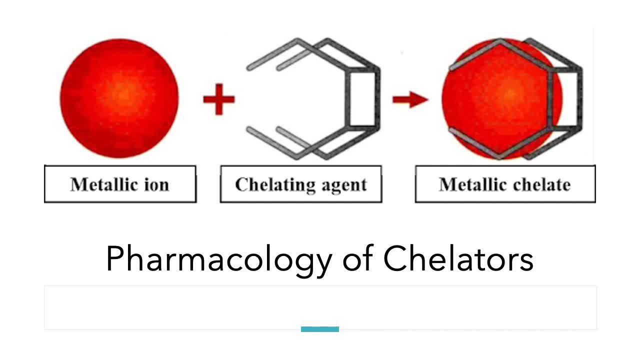 So now let's go to pharmacology of chelators, the ones that we use as treatment or antidote for metal poisoning. So the basic principle of chelators is that it binds metallic ions tightly and make them or render them water-soluble and ready for excretion. 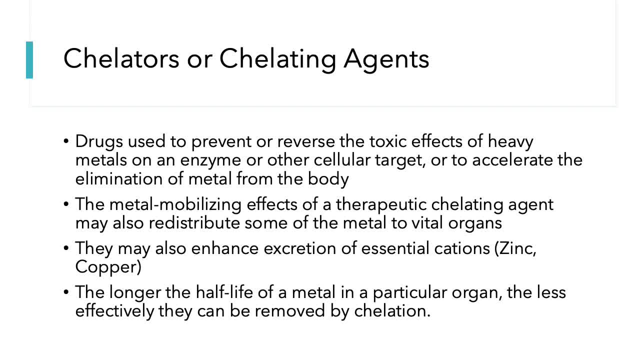 So chelators or chelating agent comes from the Greek word kela or mesothelioma, So chelators or chelating agent comes from the Greek word, or mesothelioma, So chelators or chelating agent, comes from the Greek word. 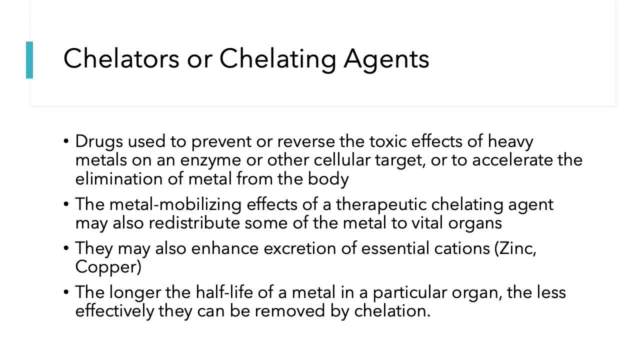 meaning crab's claw. By forming a complex with the hemi-metal, the chelating agent renders the metal unavailable for toxic interaction with functional groups of enzymes or other proteins, coenzymes, cellular nucleophiles and membranes. Chelating agents contain one or more coordinating atoms. 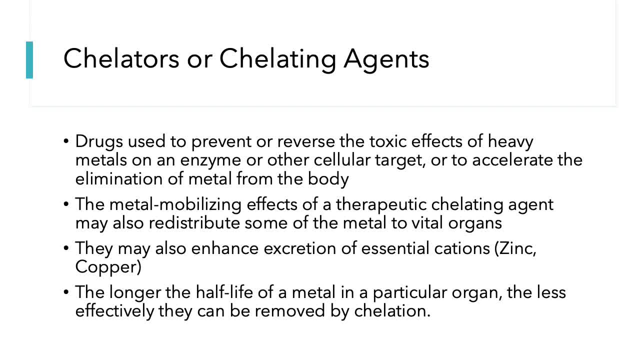 usually oxygen, sulfur or nitrogen, which donates a pair of electrons to a cationic metal to form one or more coordinating atoms. So chelators or chelating agents come from the Greek word covalent bond, So therefore making them water-soluble, ready for elimination. 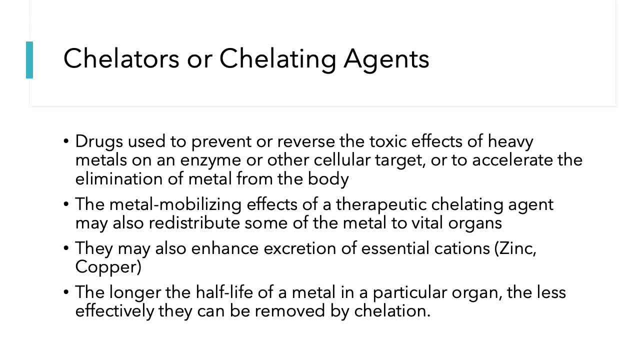 However, there are many limitations to chelating agent One. the metal metabolizing effect of a therapeutic chelating agent may also redistribute some of the metal to vital organs. Like the dimercaprol, it has the ability to redistribute mercury and arsenic to the CNS or brain, while at 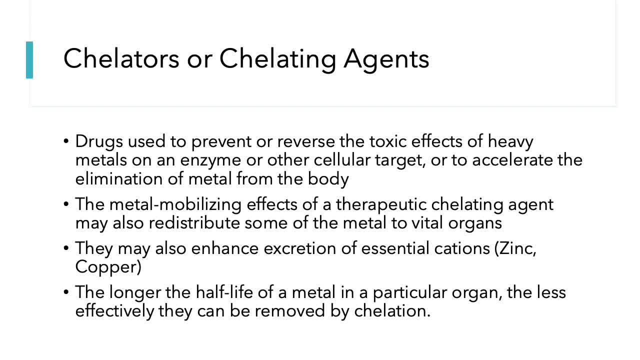 the same time it can redistribute mercury and arsenic to the CNS or brain. So chelating agents can also be added to the chelating agent Two. they may also enhance excretion of essential cations like zinc and copper: Zinc for EDTA, zinc and copper in succimer. Another one is: 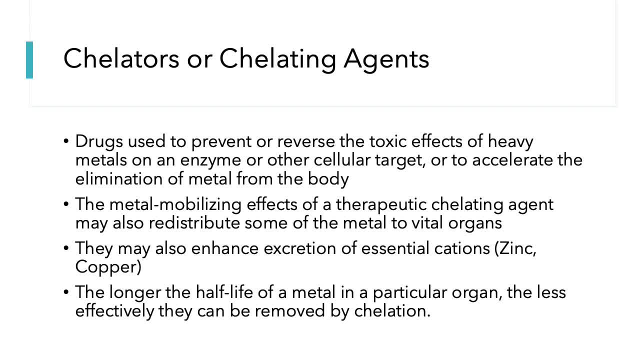 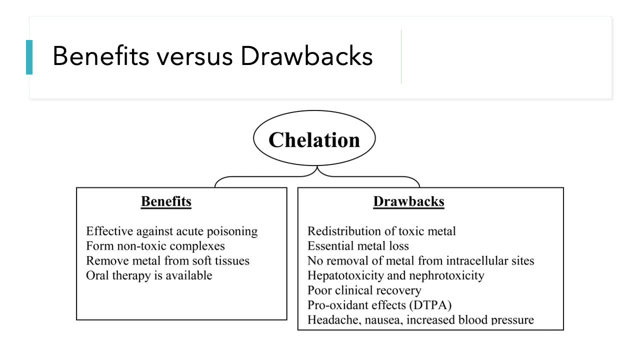 the longer the half-life of the metal in a particular organ, the less effectively they can be removed by chelation. Therefore it is best given during the acute phase of toxicity. So here are the benefits and drawbacks that I've mentioned. just a summary. 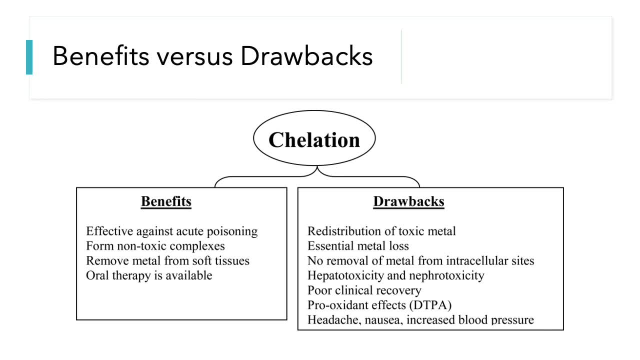 The benefits. it's effective against acute poisoning forms non-toxic complexes. more water-soluble complexes remove metal from soft tissues and oral therapy is available in some of those chelating agents. Drawback it again redistributes toxic metal to other organs of the body. 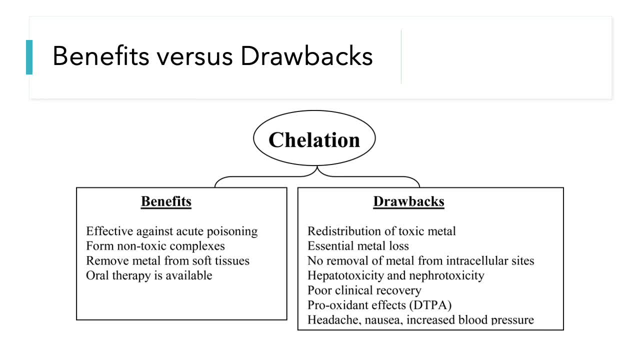 And of course, there's loss of essential metals: no removal of metal from intercellular sites. There are some limitations to some of the chelating agents. Hepatotoxicity and nephrotoxicity is a glaring side effect. Patients may have poor clinical recovery as well, depending on the phase of the treatment. 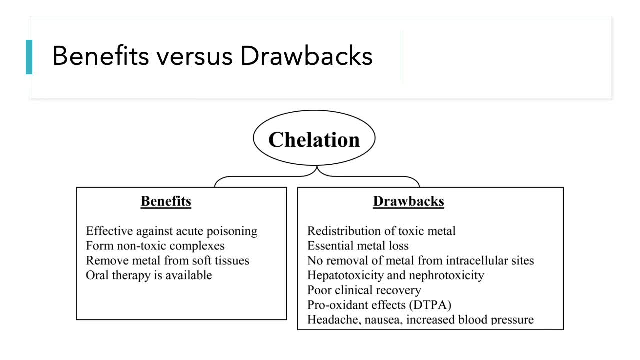 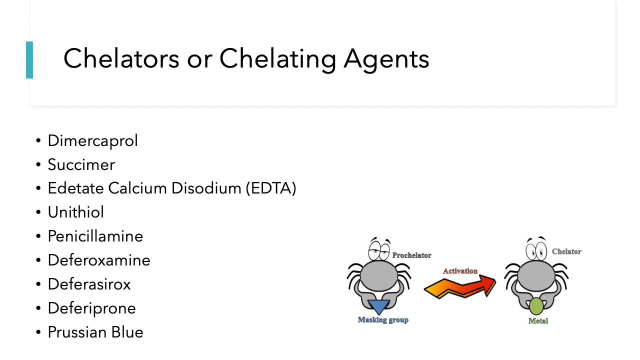 Pro-oxidant effects like DTPA, so more oxidative stress is produced, And then headache, nausea, increased blood pressure are also other side effects. So the chelators or chelating agents that we use right now are dimercaprol, succimer, EDTA- that's very famous edetate- calcium disodium. 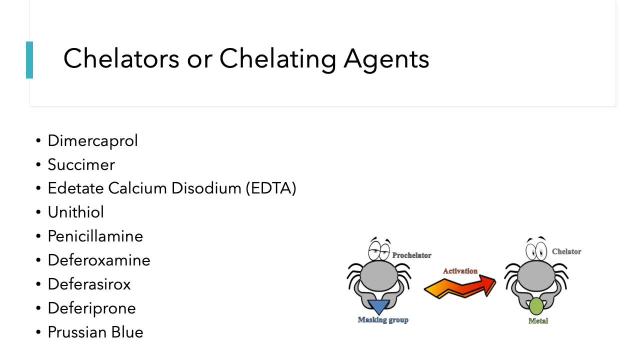 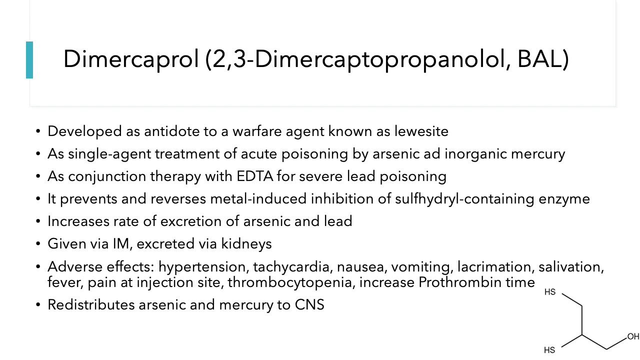 unitiol, penicillamine, a derivative of penicillin, deferoxamine and deferacerox and deferapiron. There's also what you call Prussian blue. The first of the chelating agent, or chelating agent, are dimercaprol or 2T dimercaptopropanolol. 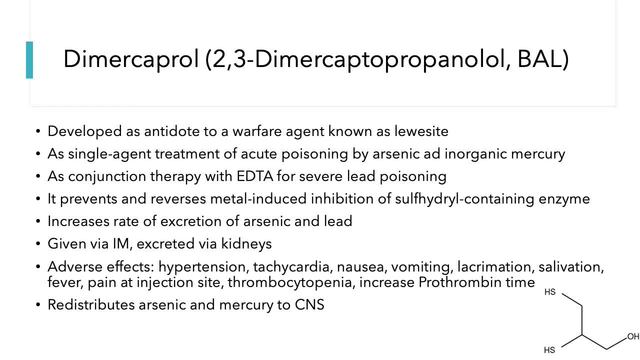 It is also known as BAL or British anti-leucite, because initially it was developed as an antidote to a warfare agent known as leucite in World War II, So it is used primarily as a single agent treatment of acute poisoning by arsenic. 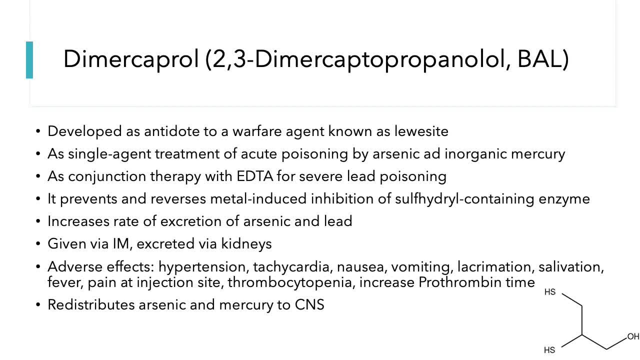 and inorganic mercury. It is also used as a conjunction therapy with EDTA for severe lead poisoning. It prevents and reverses metal-induced inhibition of sulfhydryl-containing enzyme. It increases the rate of excretion of arsenic and lead, and it's usually given via IM and excreted via kidneys. 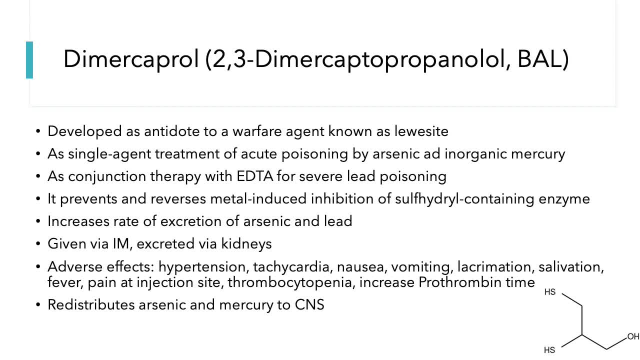 The adverse effects of dimercaprol are hypertension, tachycardia, nausea, vomiting, lacrimation, salivation, fever, pain at injection site, thrombocytopenia and increased prothrombin time. It redistributes arsenic and mercury to CNS. 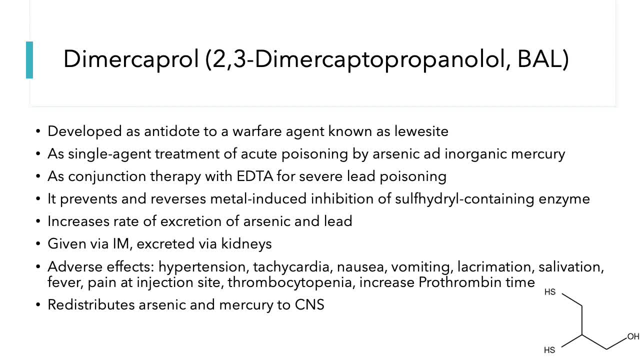 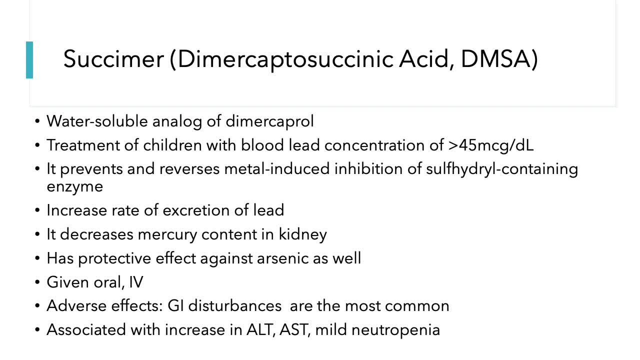 So therefore it is not advocated for treatment of chronic poisoning. Suximer or dimercaptose succinic acid or DMSA, is a water-soluble analog of dimercaprol. Its treatment of choice for children with blood level of concentration. 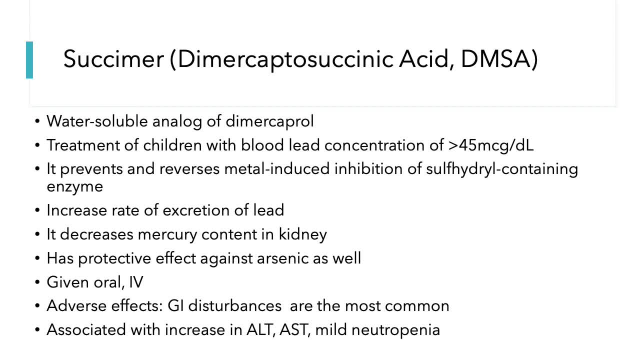 of greater than 45 micrograms per deciliter. So it prevents and reverses metal-induced inhibition of sulfhydryl-containing enzymes and increases the rate of excretion of lead. It decreases mercury content in kidneys as well. It has protective effect against arsenic. 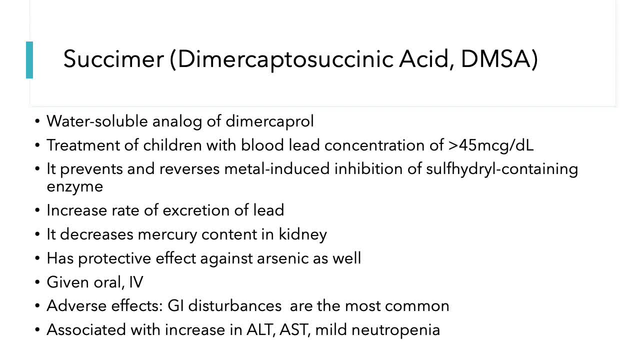 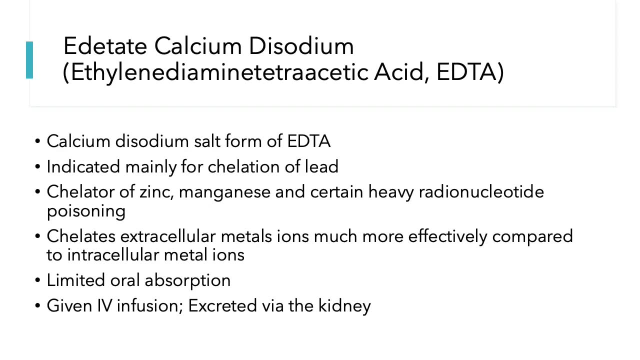 and it is given orally and via IV route. Now, Adverse effects: the most common are your GII changes or disturbances. It is also associated with increased amino transferases and mild neutropenia: Editate, calcium disodium or ethylenediamin, tetraacetic acid or EDTA. 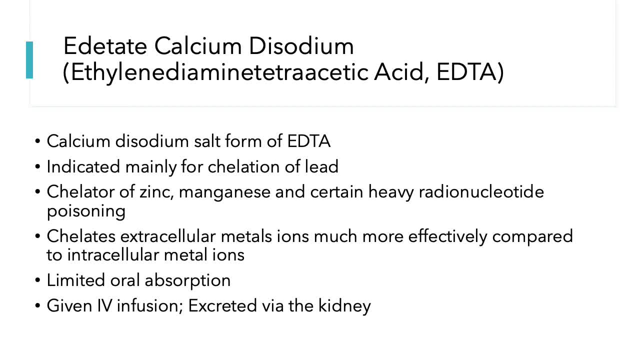 This one is very famous. It's used in your purple top to prevent coagulation of blood. In the case of heavy metals, the calcium disodium salt form of the EDTA is used because a calcium form reduces the potential depletion of calcium stores in the body, which is life-threatening. 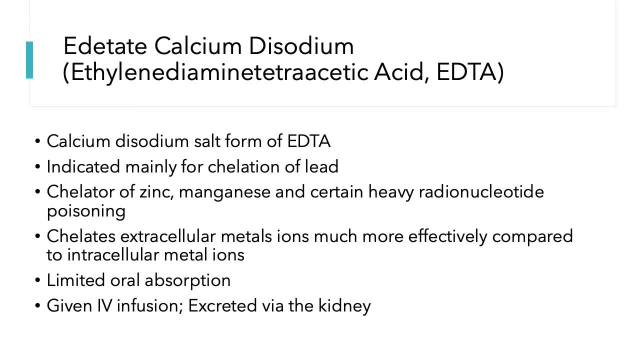 And it is indicated mainly for chelation of lead, Chelator of zinc as well manganese and certain heavy radionuclid poisoning. It has propensity. It has propensity to chelate extracellular metal ions more effectively compared to intracellular metal ions because it penetrates poorly to the cell membrane. 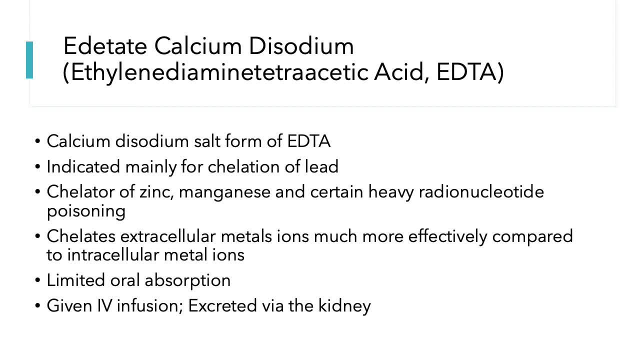 It has limited oral absorption because, first, it's highly polar And, number two, it may increase absorption of lead if it's in the gut as well. So, given IV infusion excreted via the kidneys, What are the benefits of Dynmercaptopropanosulfonic acid? 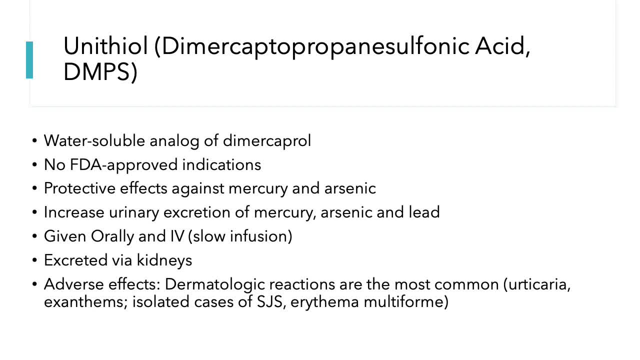 Unitiol or Dynmercaptopropanosulfonic acid, or DMPS, is a water-soluble analogue of Dynmercaprol. As of today, there are no known FDA or USFDA approved indications for these, But many studies have suggested that unitiol have advantages over IM-Dynmercaprol or oral succimer. 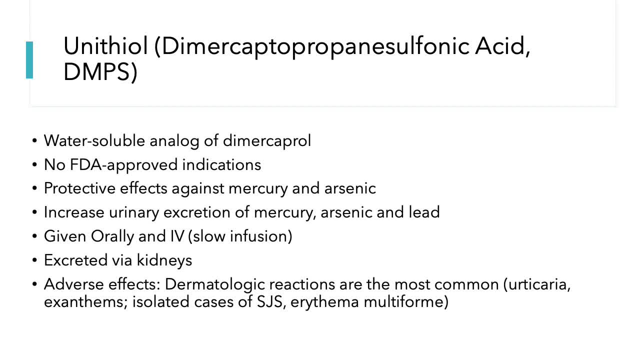 In the initial treatment of severe ulcerative colitis it is recommended to use Dynmercaptopropanosulfonic acid as the main ingredient for Dynmercaprol of severe acute poisoning by inorganic mercury and arsenic. It increases urinary excretion of 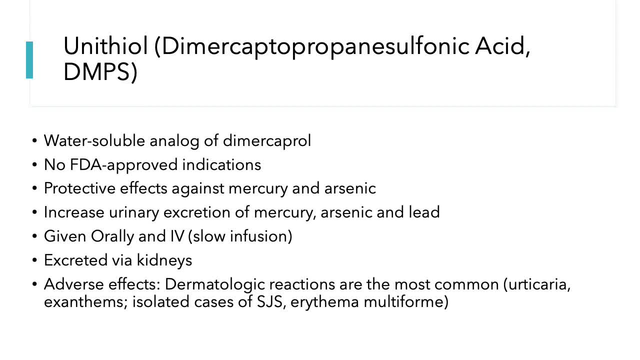 mercury, arsenic and lead. given orally in IV via slow infusion. It is excreted via the kidneys. It has low overall incidence of adverse reactions or effects and the most common forms are dermatologic reactions like urticaria exantems. Some patients have isolated cases of Steven. 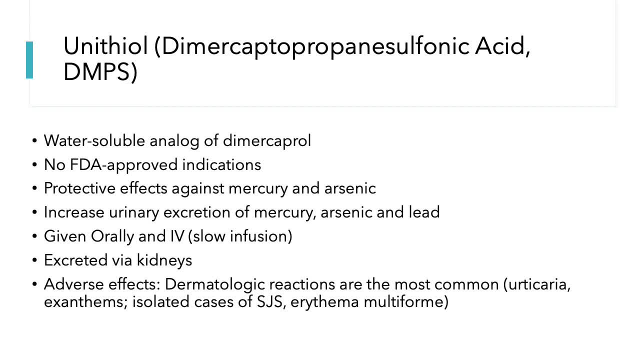 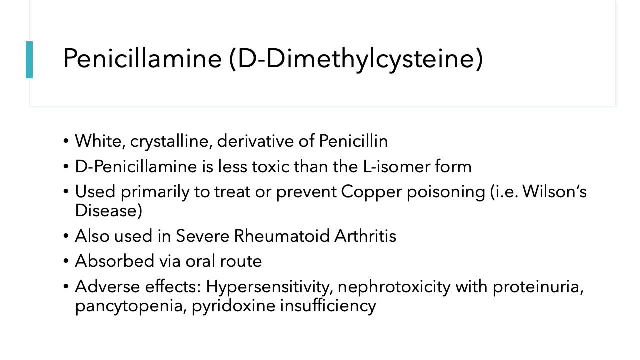 Johnson syndrome or erythema multiforme. Diphenylamine, or D-dimethylcysteine, is a white crystalline derivative of penicillin. The diphenylamine is the preferred form because it is less toxic than the L-isomer form. It is used. 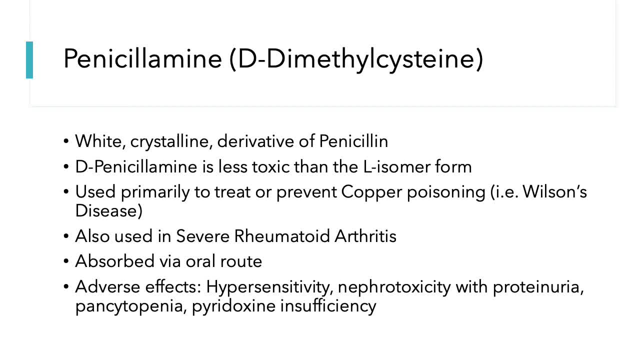 primarily to treat or prevent copper poisoning, especially in Wilson's disease. It is also used in severe rheumatoid arthritis. It is absorbed via the oral route. The first effects include hypersensitivity, neprotoxicity with proteinuria, pancytopenia and pyridoxin insufficiency. 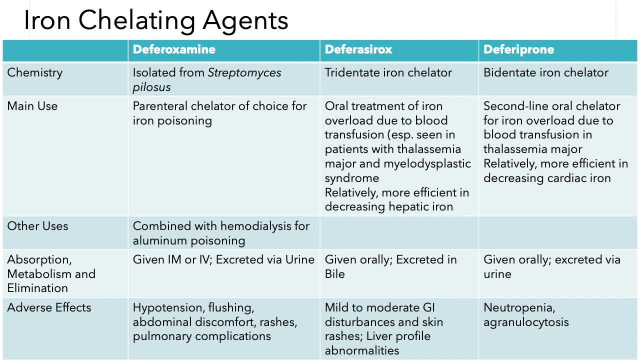 So now let's go to iron-chelating agents, or diferoxamine, difarasirox and difereprone. Let's differentiate the three. So diferoxamine was isolated from septomyces phyllosus. The main use of this is parenteral. It is used to treat or prevent cancer. It is used to treat or prevent. 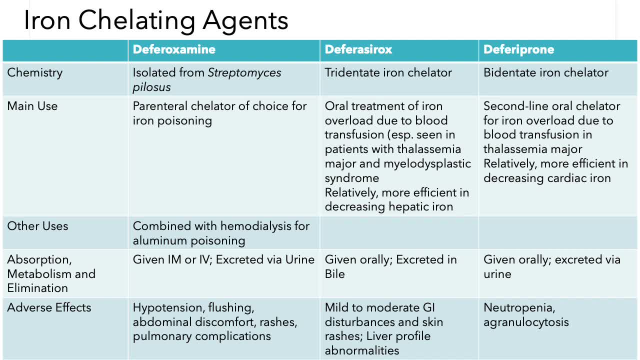 cancer. It is also used as a parenteral chelator of choice for iron poisoning And other uses. when combined with the imodalialysis is good as well for aluminum poisoning. The absorption route it's given via IM and excreted via the urine. The adverse effects include hypotension, flushing. 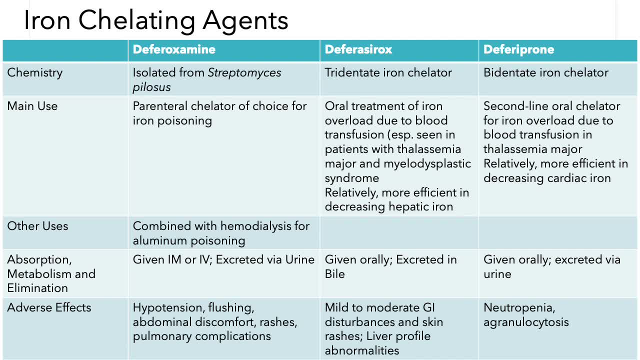 abdominal discomfort, rashes and pulmonary complications. Diferasirox is a tridentate iron chelator. It is mainly used to treat or prevent cancer. It is also used for the treatment- oral treatment- of iron overload due to blood transfusion, especially seen. 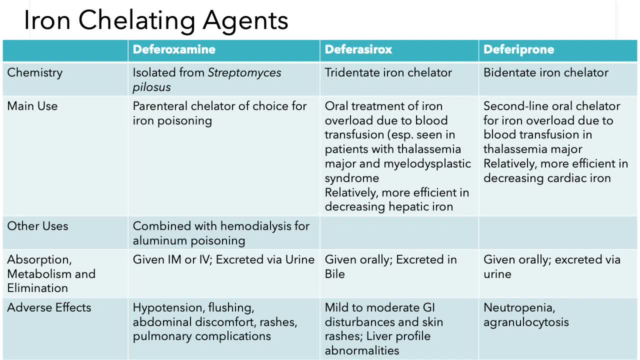 in patients with thalassemia major and myelodysplastic syndrome. It is relatively more efficient in decreasing hepatic ion compared to difereprone. It is given orally excreted via bile. It produces symptoms like mild tumultuous GI disturbances, skin rashes. 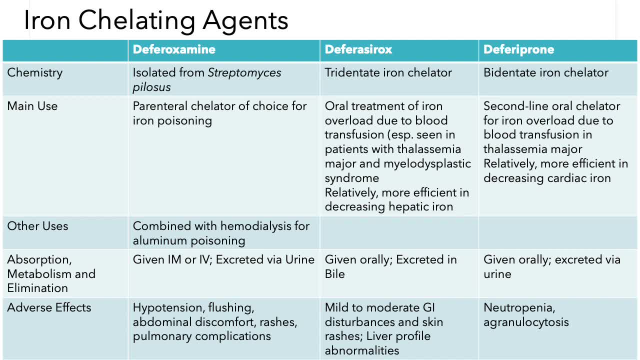 and some liver problems. It is also used to treat or prevent cancer. It is also used to treat or prevent cancer. Diferasirox is a tridentate iron chelator. It is mainly used as a second-line agent for iron. 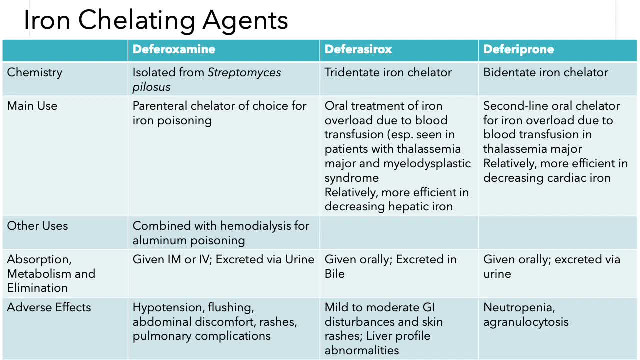 overload due to blood transfusion in thalassemia major. Relatively it has more efficient in decreasing cardiac iron compared to diferasirox. It is given orally, excreted via urine and has side effects of aminotransferases. It is mainly used as a second-line agent for iron overload due to blood transfusion in thalassemia major. 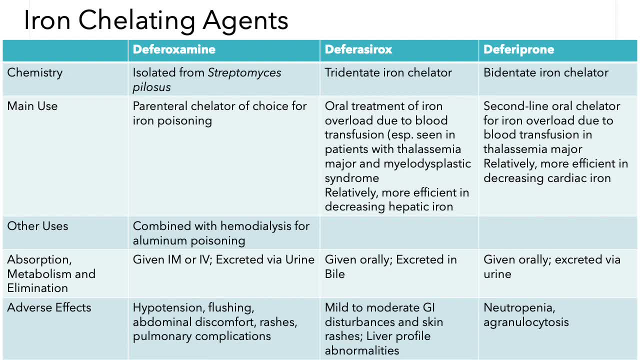 It is mainly used as a second-line agent for iron overload due to blood transfusion in thalassemia major. It is mainly used as a second-line agent for iron overload. It has more efficient in reducing트를orocytosis. It is more efficient in removing hyperacidosis due to ibuprofen. and. 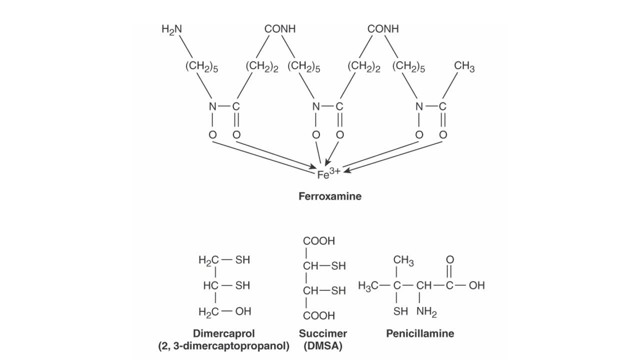 So these are the chemical structures of the several chelators that we've discussed. Ferroxamine or ferioxamine without the chelated iron is what you called diferoxamine. It is represented here to show the functional groups. The iron is actually held in a cage system. 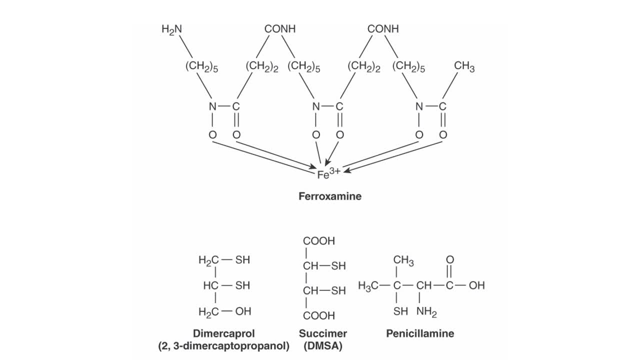 mimicking a crab-like claw. The structures of the chemical structure of the several chelators that we've discussed are the gut and the viral cell system, rows of ossuary and various other. The structures of the in vitro metal chelator complexes for dimicaprol, succimer, penicillamine and eutentile are not known and may involve the formation of mixed disulfides with amino acids. 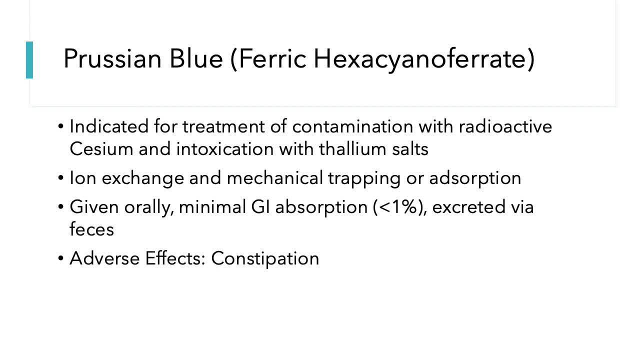 The last that we're going to discuss is your fusion blue or ferric hexacyanopherate. It is indicated for treatment of contamination with radioactive cesium and intoxication with thallium salts. This was approved mainly because of concern over terrorist use of the radioactive dispersal units called 30-bombs.